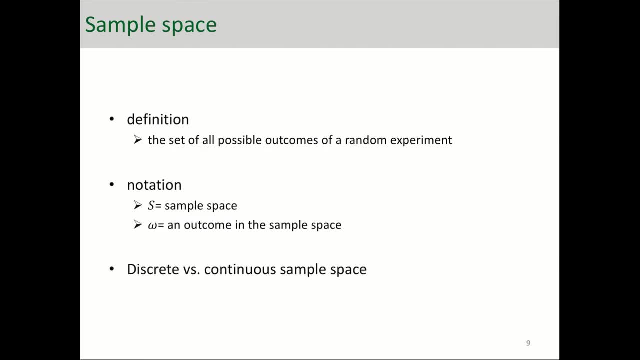 Well, there are different random experiments for a reason, and that is sample space. Their sample spaces are different. What is a sample space? Well, sample space is a set of all possible outcomes of a random experiment. When you think about flipping a coin, the sample space of that experiment is whether you obtain heads or tails. 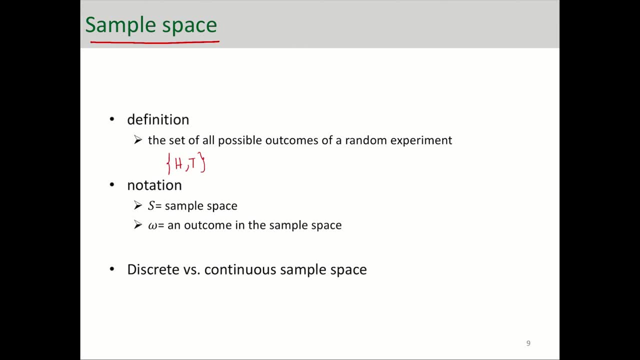 That is the sample space of flipping a coin once. At this point I want you to think about what is a sample space of flipping a coin twice, which makes it a different random experiment than flipping a coin once. The sample space is probably different. 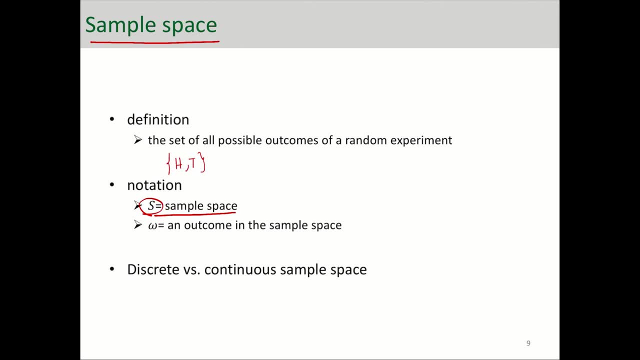 The way that we show sample space with this letter capital S. So this is how we show sample space. Sample space can be discrete or it can be continuous. What is the difference between these two? Discrete sample space is when The outcomes in the sample space are countable. 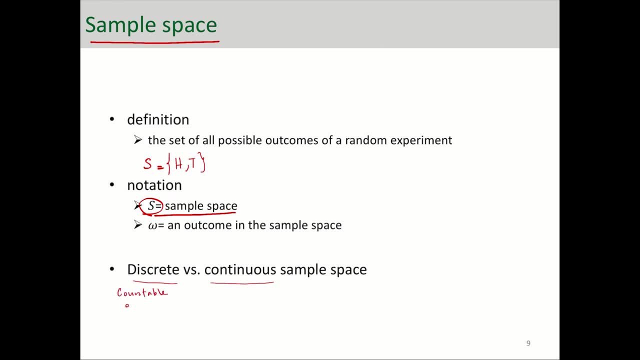 So countable outcomes. But continuous sample space is when the outcomes are not countable, So non-countable outcomes. Well, when you think about flipping a coin, once the number of outcomes are countable- One, two- The number of outcomes can be infinite, but countable. 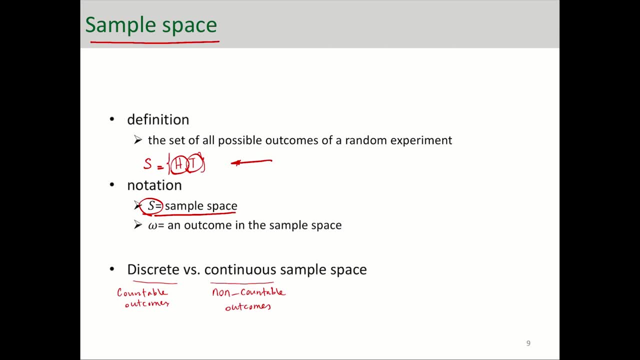 So that's a possibility. You have infinite countable outcomes and that's a discrete sample space. But when the sample space is non-countable, just like, let's say, human height, The height of us humans is a continuous spectrum of numbers. 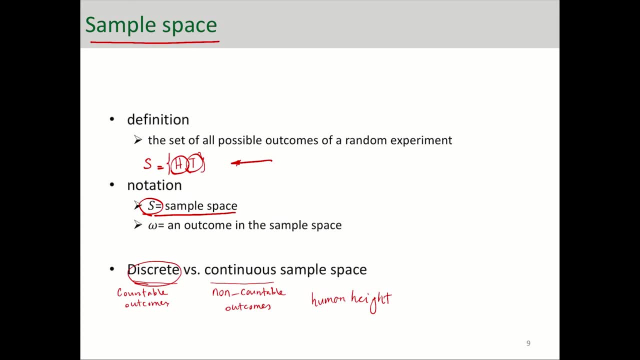 Between each two numbers, there are infinite numbers possible. That's why it's a continuous sample space. So that's the difference between discrete and continuous sample space. So, as we said, flipping a coin, the sample space is heads and tails And I want you to pause the video and think about the sample space of flipping a coin twice. 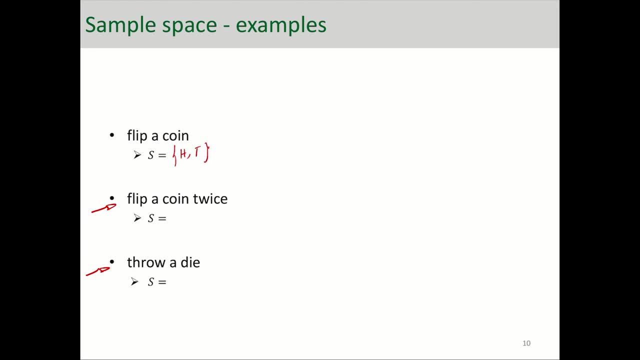 and throwing a die For flipping a coin twice, there are four different outcomes. So the sample space contains those four Heads: heads, tails, tails, head and tails, tails. So four different outcomes in that sample space. When you're throwing a die, what is the sample space there? 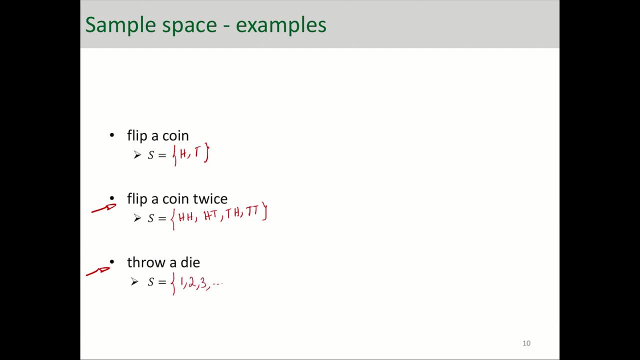 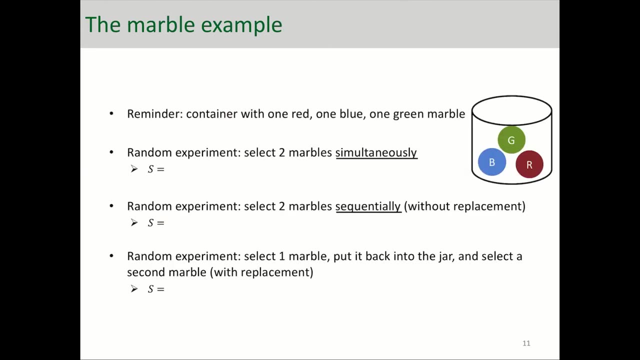 It is one, two, three, all the way to six. Six different outcomes in that sample space. Let's look at another example. This one is a little bit more difficult and I want you to pause the video and work on this slide. 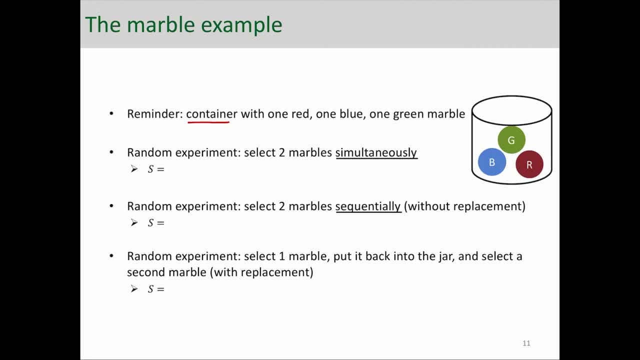 So let's consider a container with one red, one blue and one green marble, as you can see in this picture, And the random experiment here is selecting two marbles simultaneously. So basically, you put your hand in the container and you grab two marbles. 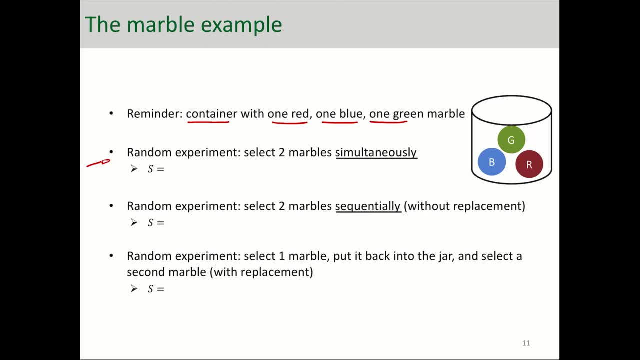 What outcomes can happen? Well, you might grab these two, you might grab these two, and you might grab these two. That's all the three possible outcomes, right? So I'm going to write red blue. I'll say green red and green blue, right? 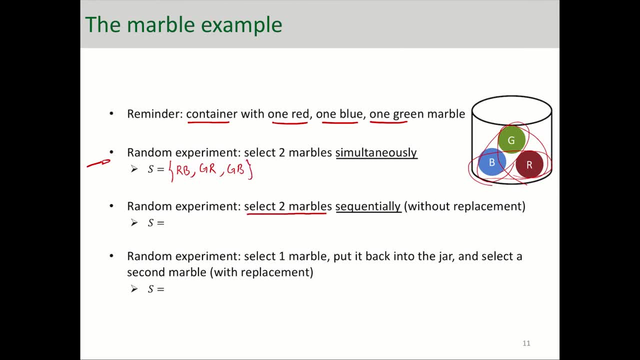 The other experiment is selecting two marbles sequentially, without replacement. It basically means that you put your hand in the container, you grab one marble and then with the other hand, you grab another marble. It's not at the same time, it's sequentially. 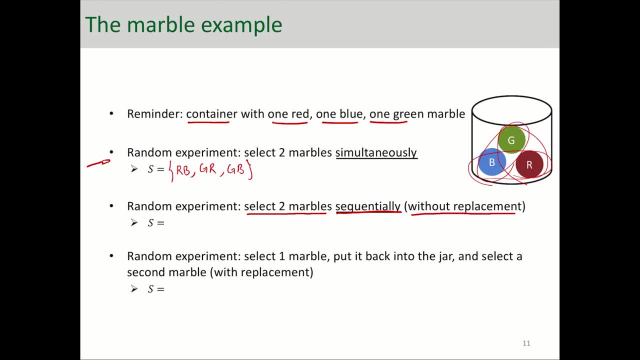 And it's without replacement because you don't put back the first marble that you grab. So what is the sample space here? Well, what happens here is that the order matters. The order of marbles that you grab here matters. Basically, you can have blue-red, you can have red-green and you can have blue-green.